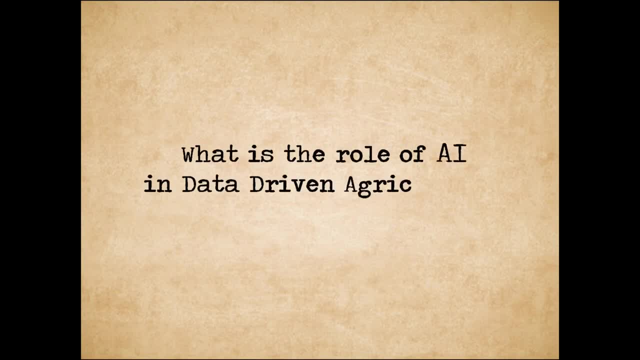 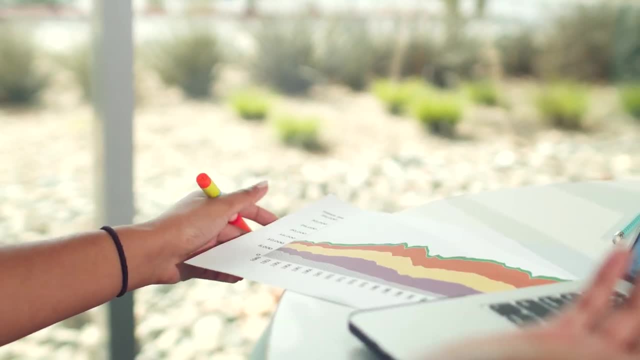 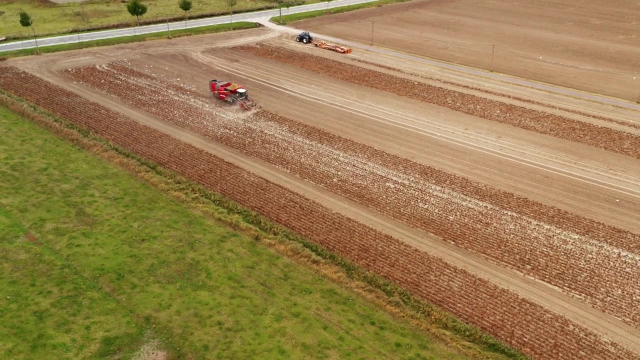 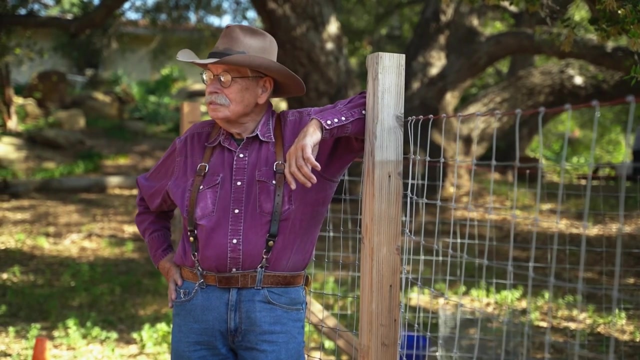 Data-driven agriculture means maximizing the insights from your data towards your return on investment, but this is easier said than done. Agricultural activities, and specifically farming, are complex processes with high number of variables involved. As a result, farmers have to evaluate many uncertainties before making a decision. Thanks to advances in precision, 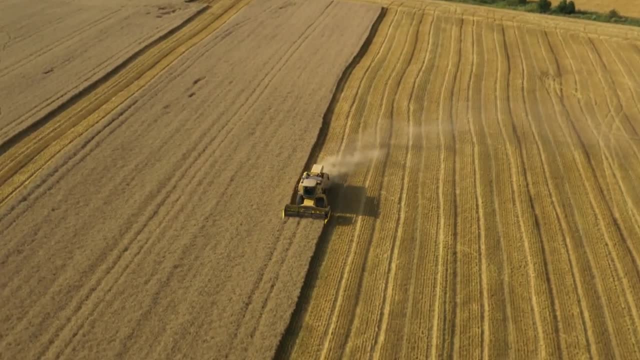 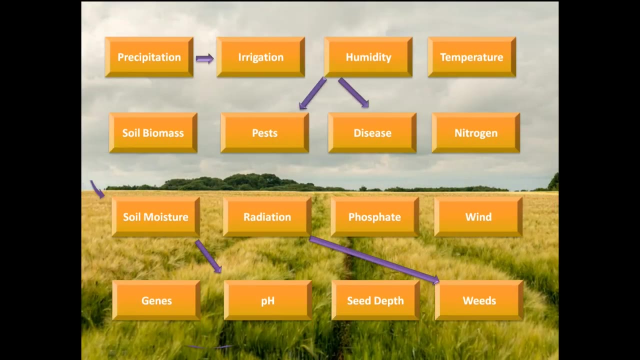 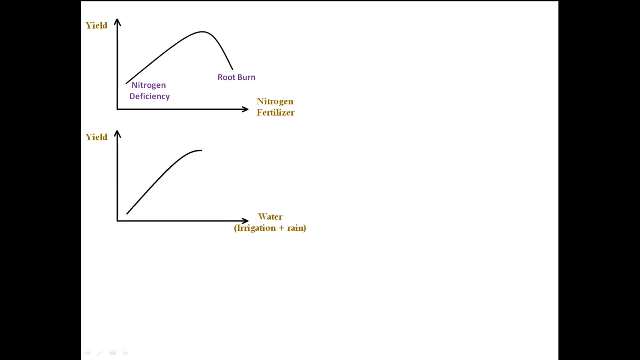 agriculture. different types of data are collected from the farms. Data-driven farming is not only about finding the way these inputs affect outputs of farm, but also the complexity of interactions between these variables. Let's show the challenge of extracting insight from farm data with a simple example: The role of nitrogen, fertilizer, water and herbicide on. 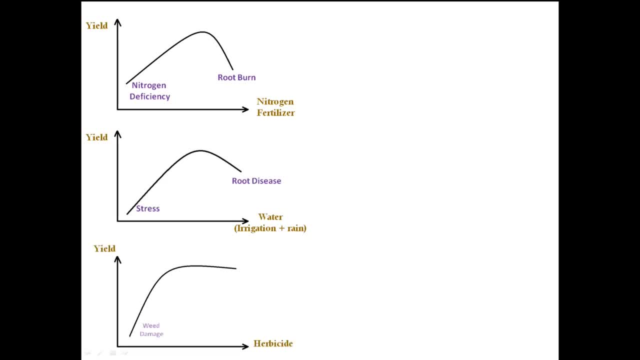 yield is known and pretty much established. Having all other factors unchanged, you can find the optimum amount of each to maximize the yield. However, having all other factors unchanged is an assumption that never happens in farming. In reality, these variables change simultaneously and each one is affected by others. Rain and irrigation could wash. 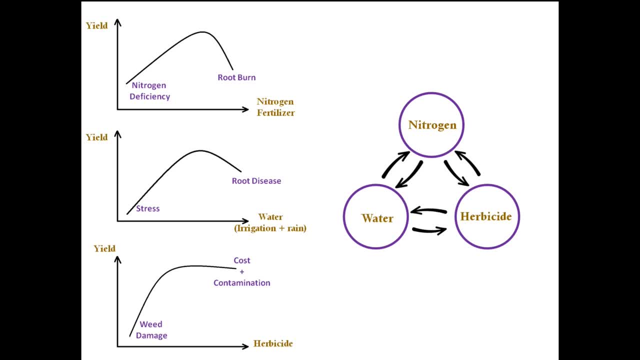 down nitrogen and herbicide. Nitrogen and weeds affect the uptake of water by plants. Weeds consume part of nitrogen out of soil and part of nitrogen out of the soil. Nitrogen and weeds affect the uptake of water by plants. Weeds consume part of nitrogen out of soil. 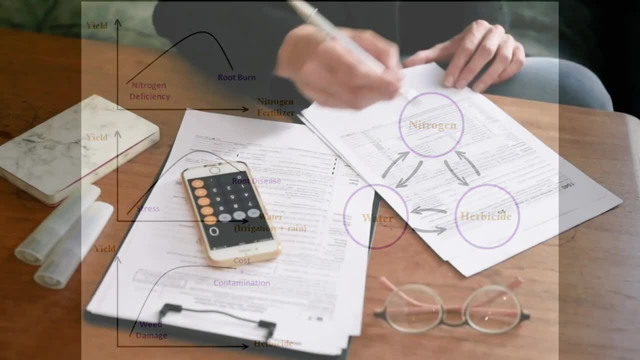 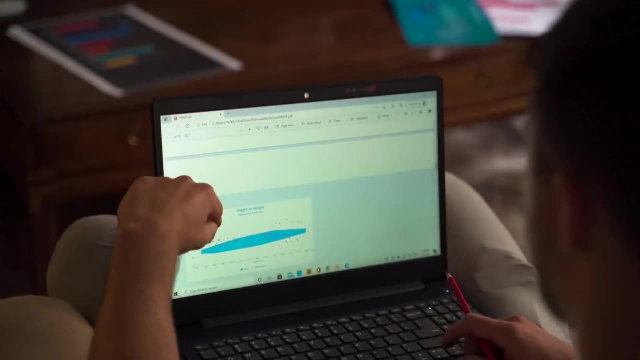 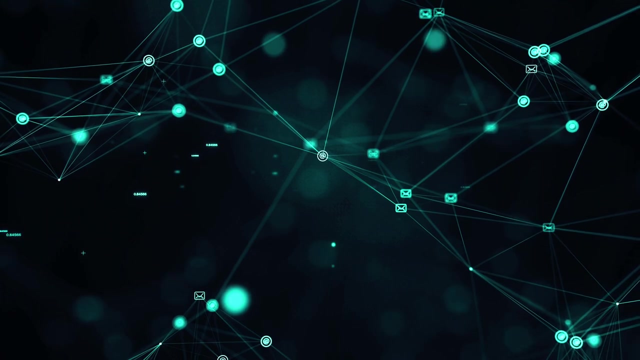 and nitrogen affects the efficiency of herbicide. There are many more factors involved in farming and, as a result, data-driven decision is not a straightforward task, even having all the data collected. While complexity in data can overwhelm the human mind, machine learning algorithms are structured to deal with it effectively. These algorithms are designed. 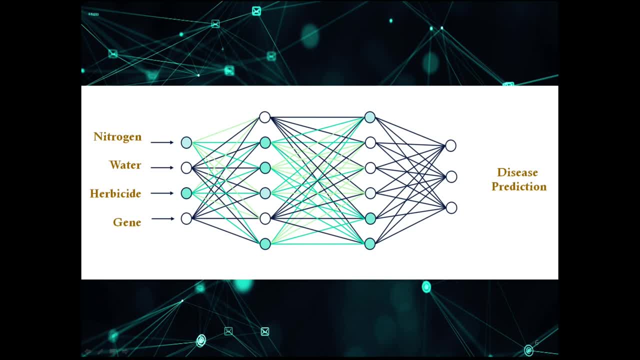 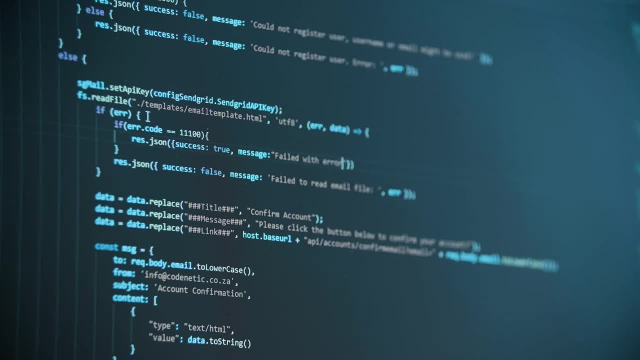 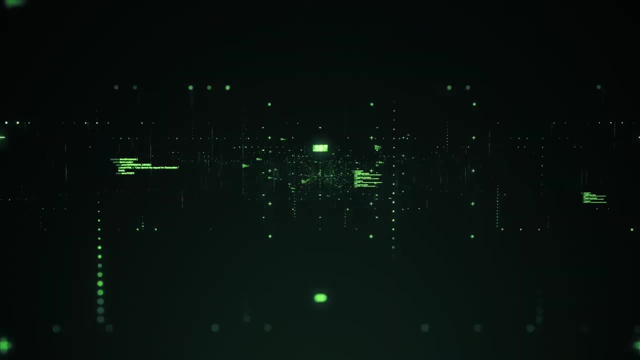 to find hidden patterns in data and predict outcomes, which leads to data-driven decision decisions that are proactive rather than reactive. Training, a reliable machine learning model is at the heart of any complex data-driven agriculture. This leads to the next phase, which is translating the insight from artificial intelligence to an actionable intelligence. 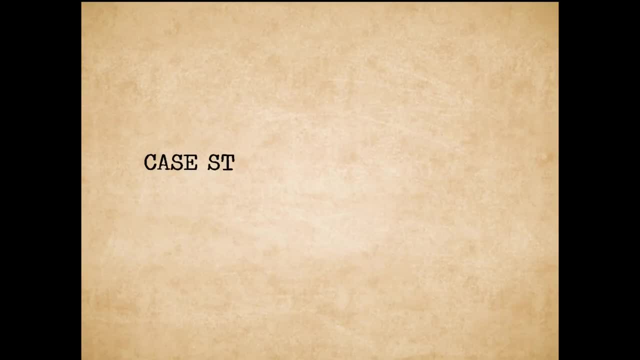 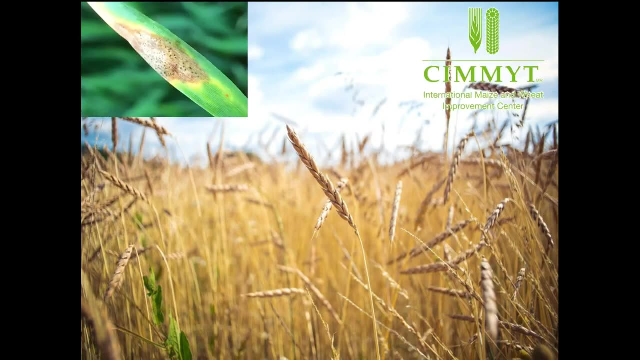 where decisions could be made upon it. Well, where does that answer the question? We obtained wheat farms data from CIMMYT, fed part of the data into the machine learning model to train it and use the rest of the data to test the reliability. 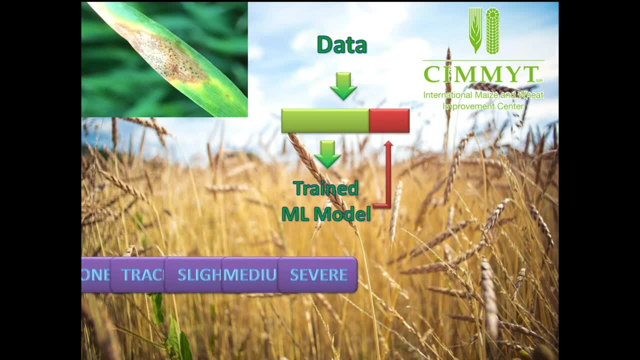 of trained model. The objective is to predict severity of foliar diseases in wheat farm before it occurs. Severity was quantified based on extent of damage, from none to severe. Our trained model could predict severity of foliar disease with 89% accuracy. 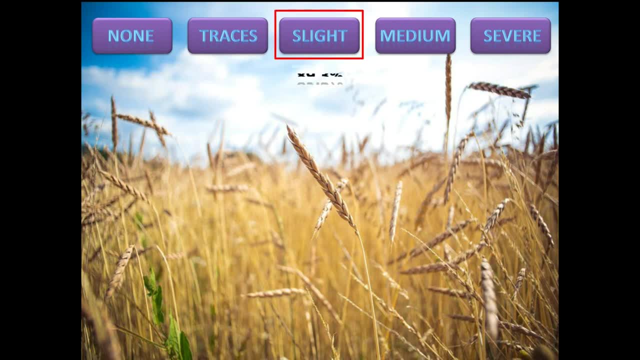 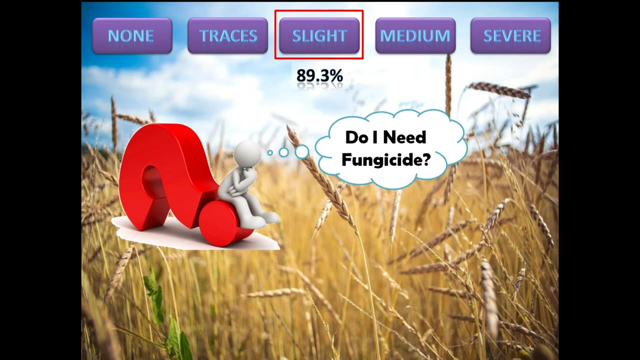 Let's say, we inform the farmer that he or she should expect a slight occurrence of foliar diseases in the coming weeks. Based on this new piece of information, the farmer evaluates whether or not they should pay for fungicides this farming season. This is where data driven decision takes place. 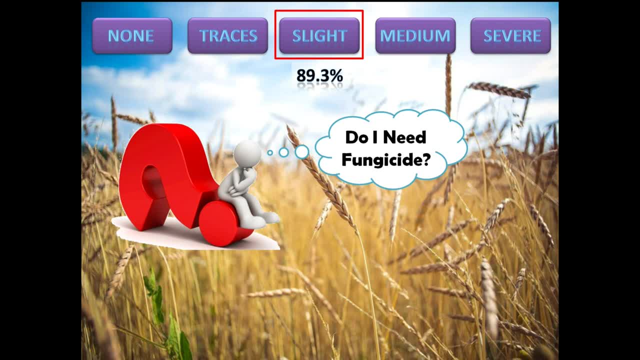 It is to make the best of the information you have, even though there is uncertainty around that. One side of the equation is the cost associated with purchasing and applying fungicides. The other side of the equation is the yield loss because of a occurrence of foliar disease. 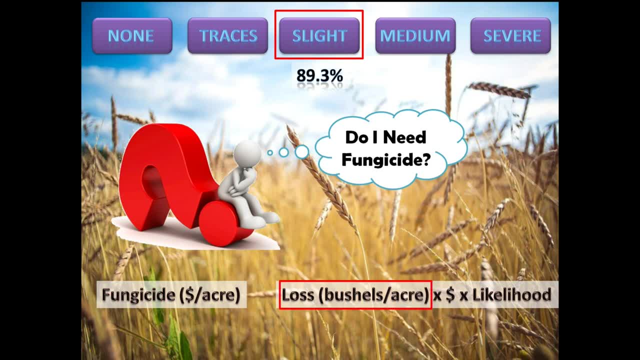 is. This can be estimated from historical data, multiplied by dollar value of that loss, multiplied by how likely it is that to happen, which comes from machine learning model. Comparing two sides of this equation leads to an informed decision. This was a simplified scenario and farmers have to evaluate more factors before making. 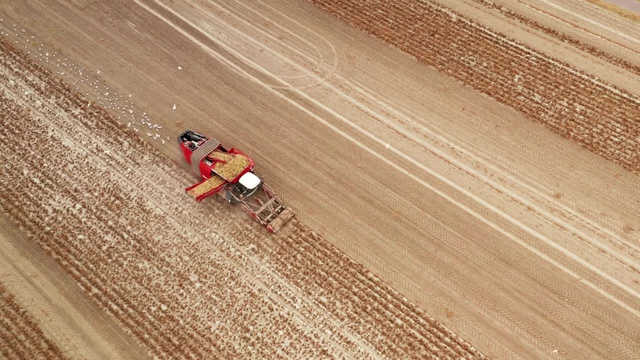 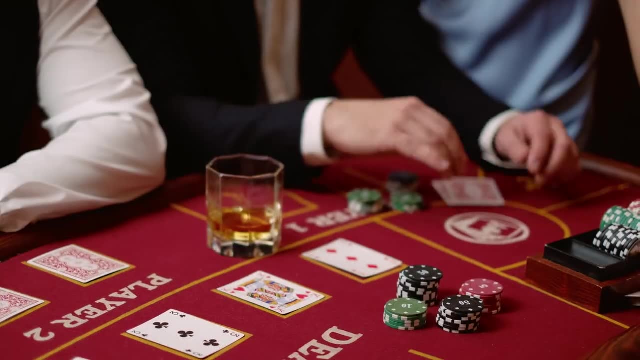 big decisions, but this shows how extra insights derived from artificial intelligence could help a farmer to turn on the machine. The answer is that the farmer is going to have a lot of fun in the future, Similar to a professional poker player that makes the best of available information at 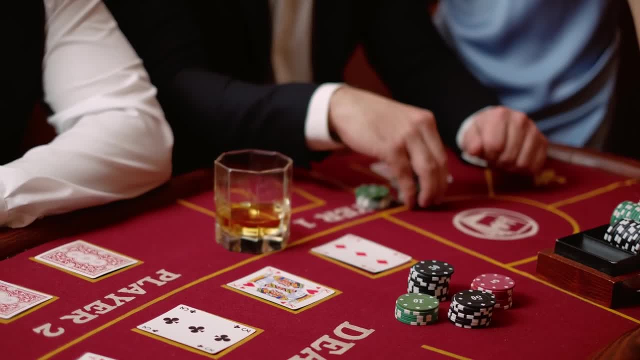 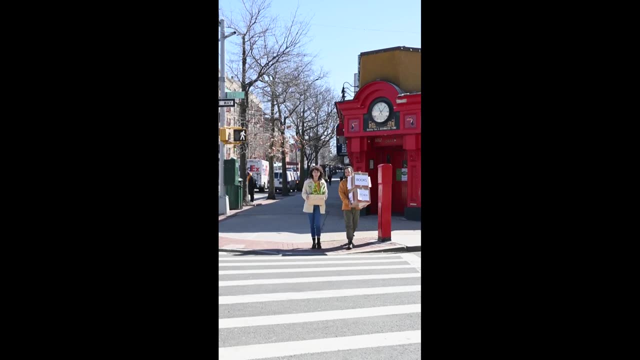 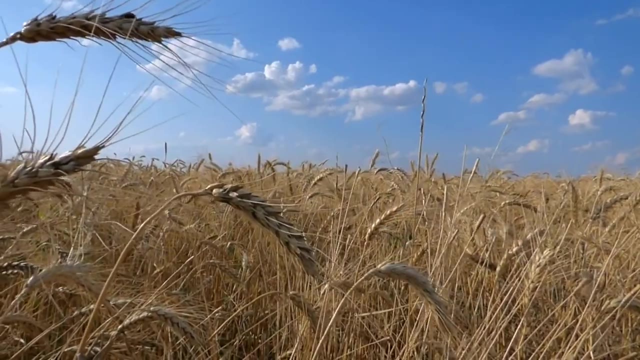 the face of upcoming uncertainty. data driven agriculture is about making the best out of your data. We all make data driven decisions on simple actions every day, with no need to use artificial intelligence. However, farming, farming data and data driven farming are not simple. 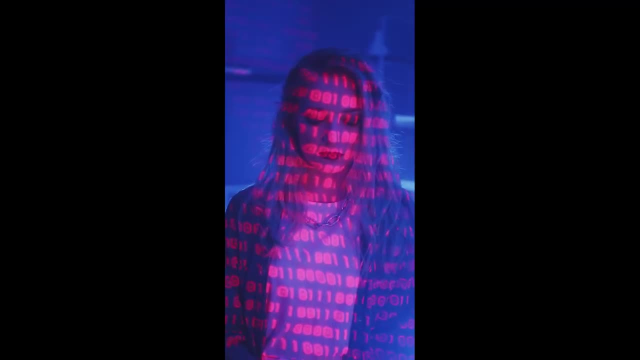 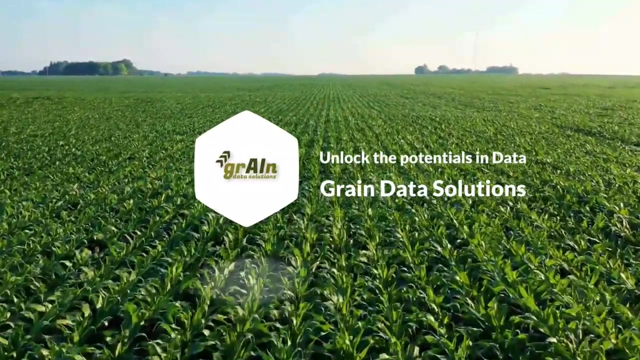 They are inherently complex, And complexity is where artificial intelligence shines. Get in touch with us today and let's discuss how actionable intelligence from AI could benefit the farming system you manage.